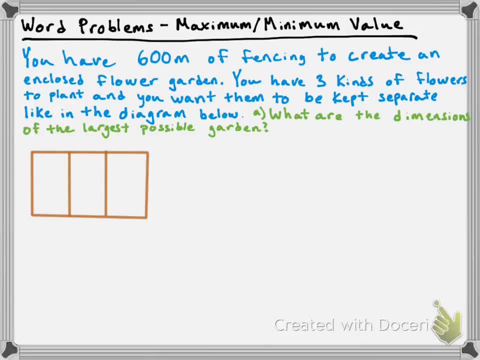 of the vertex somehow. Now, not every case is going to be like that, but many cases are going to be like that. In fact, this case is not going to be like that, but I just want to drive home the point that you're looking for the y value most of the time. okay, And we'll talk about why. 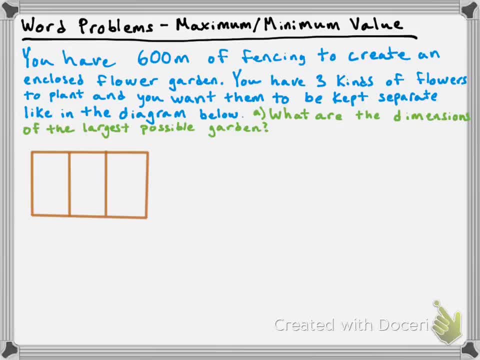 we're not doing that in this case pretty soon. So let's take a look at this question. So you have 600 meters of fencing to create an enclosed flower garden. You have three kinds of flowers to plant and you want them to be in the same place. So you have three kinds of flowers to plant. 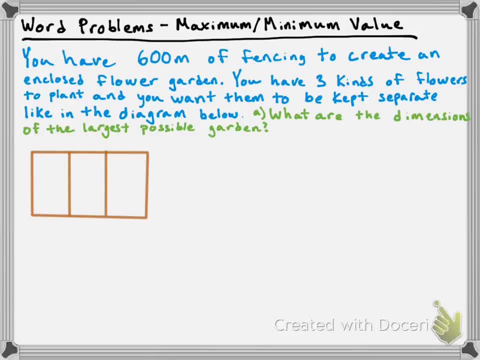 and you want them to be in the same place. So you have three kinds of flowers to plant and you want them to be kept separate, like in the diagram below. So you're going to notice that I have three different kind of sections in this diagram. I got one section right here. 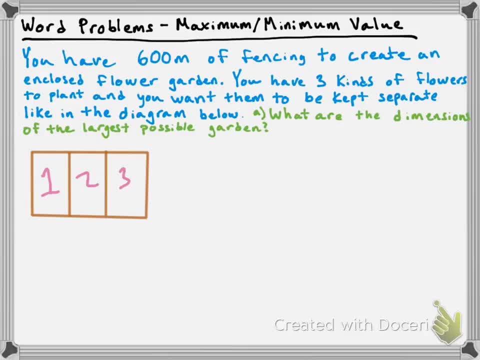 got a second section right here and a third section right here. So the idea is that in each of those sections we're going to have a kind of flower growing, okay, And you want to keep them separate. So the first question I have is A: what are the dimensions of the largest? 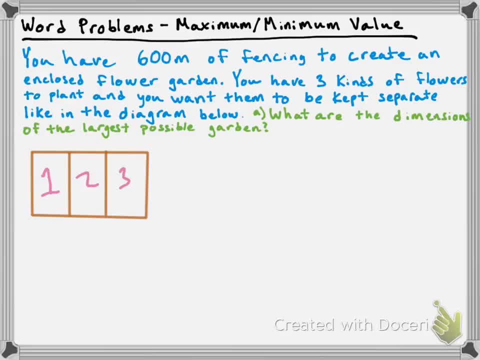 possible garden that you could make. Okay. so this is a maximum or minimum value problem, because what we're really doing is we're looking for the maximum possible area for the garden right. The largest possible garden means the largest possible area that I can. 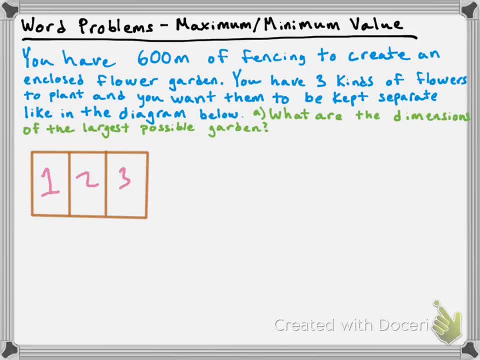 kind of cover with this garden. okay, So we are maximizing something here. We're looking for the maximum area, or specifically looking for the dimensions of the maximum area. Okay, so how do we tackle this problem? Well, first thing I want to point out to you is that this particular garden, 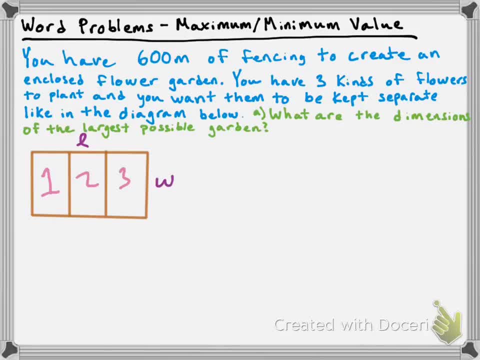 is a rectangle and, as such, it has a length and a width. okay, So the length is going to be along the top or along the bottom, The width is going to be along the sides, but I do want you to keep in. 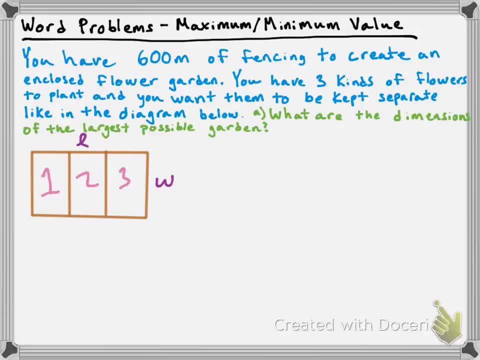 mind that, although the width is along the sides, you also have kind of two fenced sections, kind of in the middle of this big rectangle, that go up and down, and they also have the same measurement as the width on the sides. okay, So that's going to be an important detail that we're going to have. 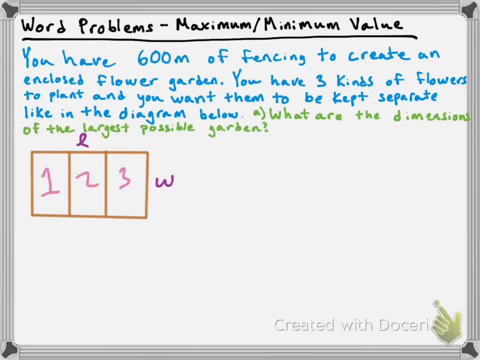 to keep in mind here. Now, why is it important? Well, remember that you have 600 meters of fencing here, and that 600 meters is going to cover the outer perimeter of this fencing, but also those two kind of sections in the middle there, right, Those two sections that go up and down, those two. 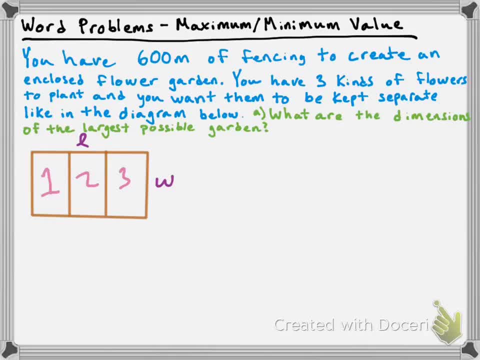 sections that go down. So that's going to come from our 600 meters of fencing as well. So let's think about how we can kind of create an equation to kind of relate the length and the width here. So let's see, So we know we've got 600 meters of fencing. Okay, so that's 600 meters of fencing. Well, that 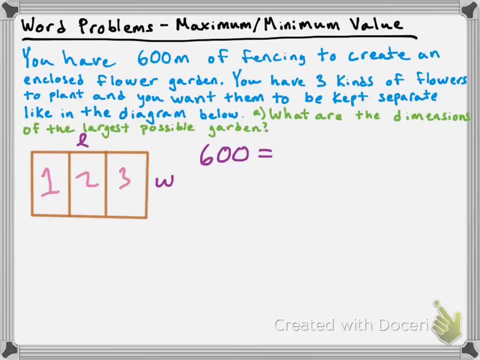 600 meters is going to be contributed by. well, let's see, we have a length of fencing along the top and we have a length of fencing along the bottom, So we have two lengths of fencing. so we're going to have: 600 is equal to two lengths. but that's not everything right, So it's not just. 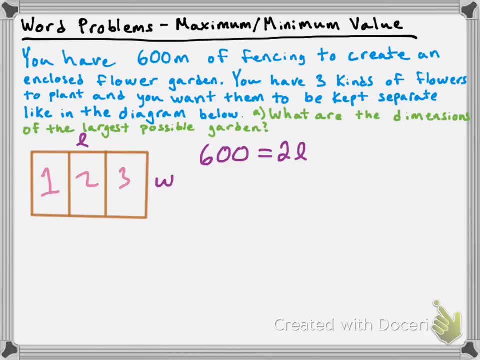 a length of fencing. it's a length of fencing along the top, And we're going to have a width on the right side, a width on the left side, but we also have those two kind of widths going through the middle right. So what we really have here are four widths that we're going to consider here, four 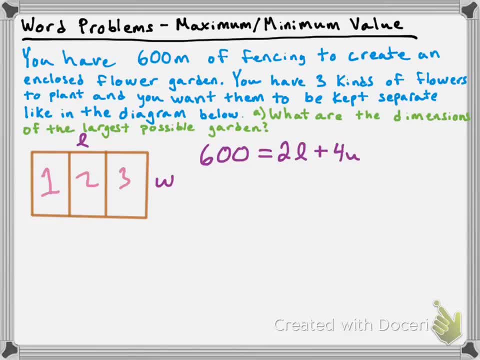 widths that are also coming from that 600 meters, So that 600 comes from the two lengths but also from the four widths. So we can kind of from that build-in equation: 600 equals the two lengths plus four widths. So if you take two of the lengths, add four of the widths, that should contribute to the 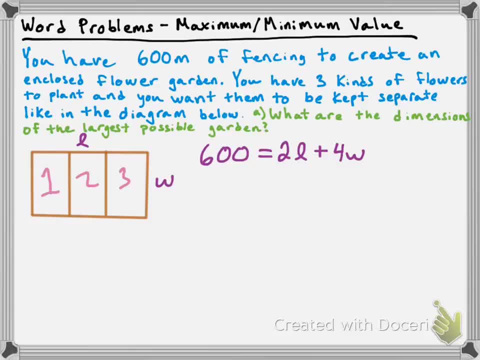 600 meters of fencing. Okay, So I'd like to take this equation and I'd like to isolate for one of my variables. It doesn't really matter which one that I isolate for, but in this case I'm going to isolate for the length, okay. 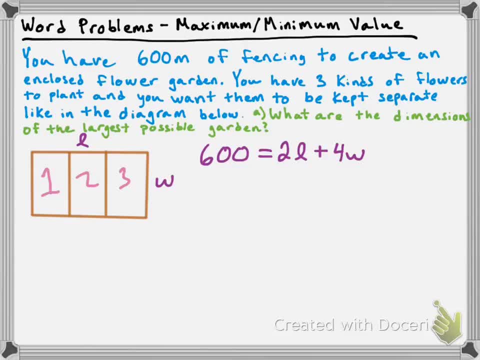 But again, it doesn't matter which one you isolate for, okay. So to isolate for length, that means you're going to have to subtract out four w from both sides. So when I do that I'm going to get 600 minus four w is equal to two l, okay. And then of course I'm going to need to divide by two. 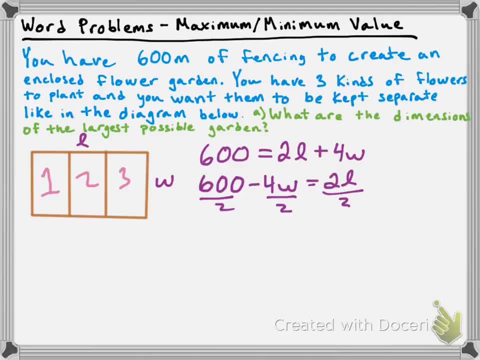 okay, So I'm going to divide everything by two, okay, And let's see. So 600 divided by two is going to be 300, negative four w divided by two is minus two w, and then two l divided by two just gives me. 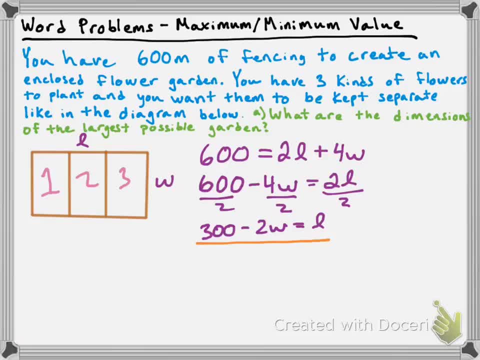 l. okay. So now I have an equation for my length that's been completely isolated for okay. So I have an expression that relates my length in terms of my width. Now, what this means is that if I know the width of this garden- okay, that gives me the maximum possible area- then I can calculate the length. 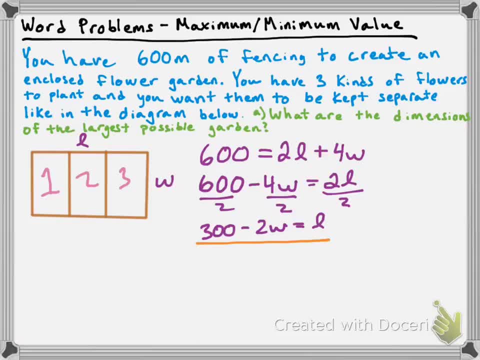 by just substituting the width in. So the next goal of this question, the next kind of immediate goal, is to find out what the width is That's going to give me the biggest possible garden, the biggest possible area. So if I'm looking for the 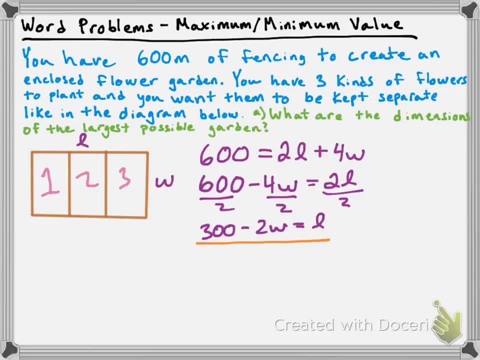 biggest possible area. that means I need an equation for area that I'm going to maximize. Now, if I'm going to maximize it, that's kind of. that implies there's going to be a maximum value and that kind of tells us that the equation that we're going to get for area is going to be it's going to be a quadratic one. 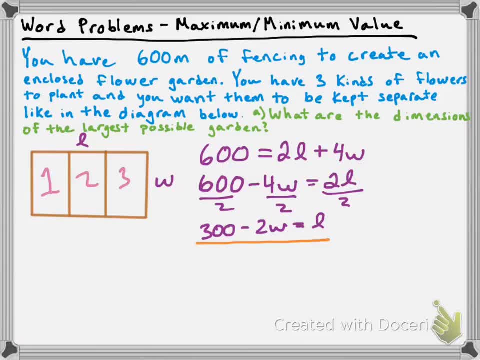 when we do this correctly. okay, It's going to be quadratic and, specifically, it'll be one that opens down, So we're going to see that in a moment. So I want you to remember that the area formula for a rectangle is just going to be this: 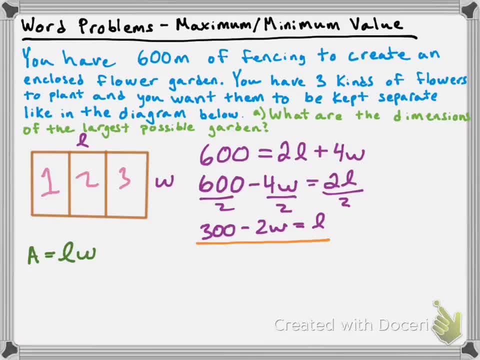 It's just: a is equal to l times w. Okay, cool. So next thing I want to do is just to make the equation look a little bit neater and a little bit more like what you're used to. I'd like to make just a quick. 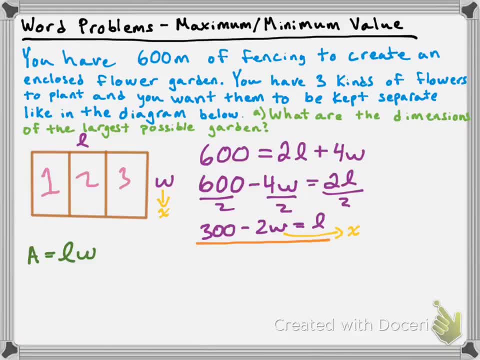 variable switch here, right. So I want to pretend that instead of w we're going to be using x. So x is going to represent our width for our equation. okay, But it still represents our width. So that means that width is x and instead of 300 minus 2w as the formula for our length, we're going to have 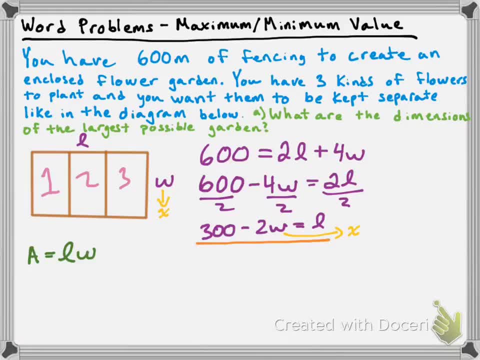 300 minus 2x. So let's make some substitutions then. So instead of l in my area formula, I'm going to substitute my expression for length that we just found by isolating for l, and that's going to be a is equal to 300 minus 2x. 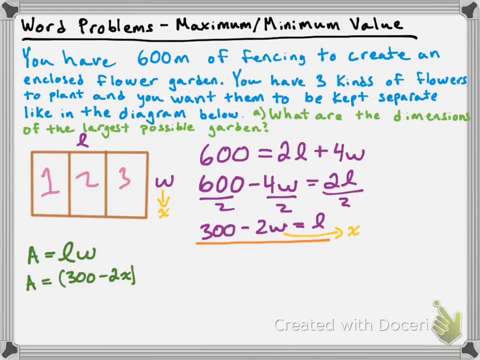 So, again, we switched out w for x instead, okay, And then I have width, which we just replaced with x, So that's the second thing in here. So I'm going to multiply that by x. Okay, cool, So I have 300 minus 2x times x. 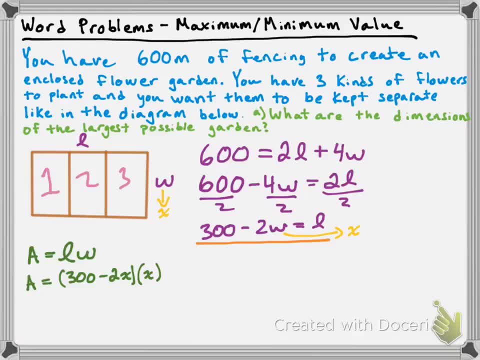 That's a formula that represents the area of my garden, given my width, which, again, we're calling x right now. Okay, so what I'm going to do now is I'm going to multiply this x into my bracket, So I'm going to distribute it. 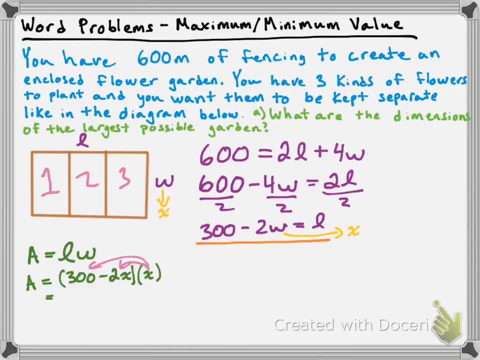 Let's see what happens when I do that. So I'm going to have 300 times x and that's going to give me 300x. and then I have x times negative 2x, which gives me minus 2x squared. So I get 300x minus 2x squared, okay. So you're going to notice that is a quadratic. It's just written that way. So I'm going to do that. So I'm going to do that. So you're going to notice that is a quadratic. It's just written that way. 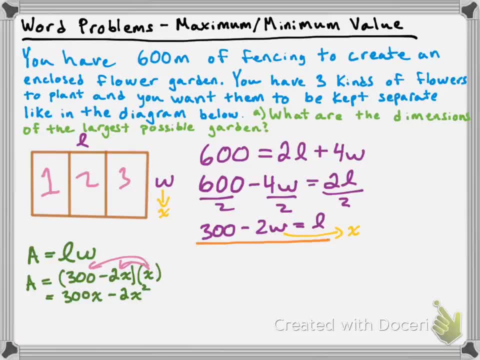 A little bit out of order compared to what you usually would do. So usually in standard form that x squared term would come first, so before the 300x. So what I'm going to do is I'm going to just kind of rearrange them. 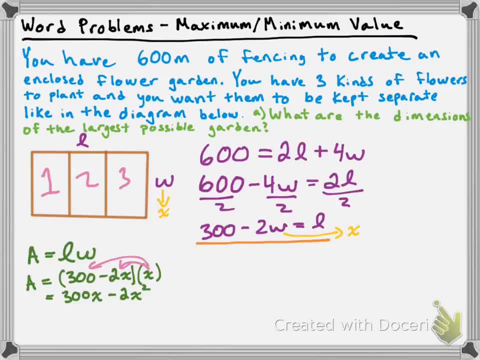 So you've got to keep in mind that the 2x squared is actually minus 2x squared. So if I move that, I'm going to have minus 2x squared and since the 300x is positive, I'll have plus 300x. 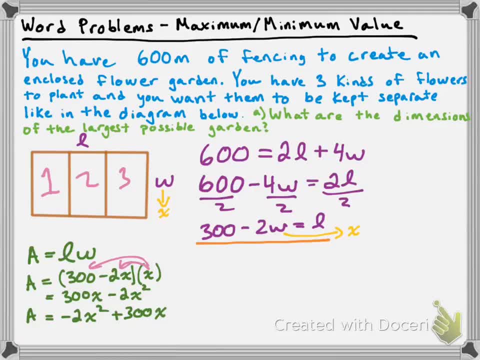 So I get a is equal to negative 2x squared plus 300x. Now that's not exactly like standard form, you'd think, because you know we usually have a C value at the end, But in this case we kind of do the same thing. 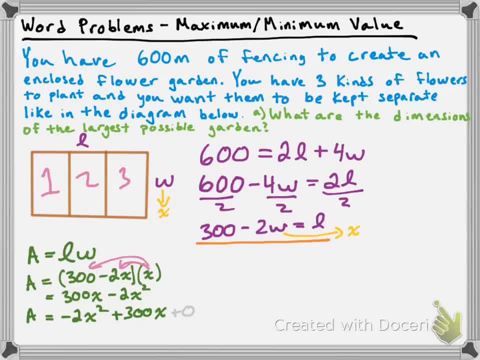 In this case, we kind of do have a c value. It's just going to be plus 0.. So our equation is: a is equal to negative 2x squared plus 300x, but there's a plus 0 at the end that you can think of as being the c value. 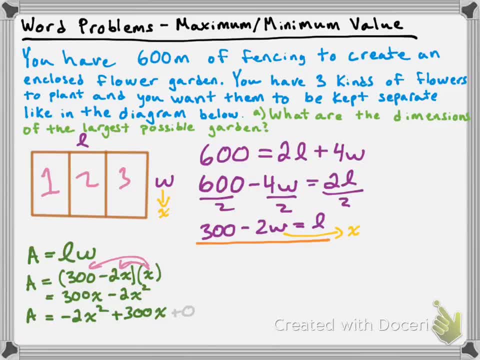 Okay, so this is the formula for the area of my garden and the goal is to find the dimensions for the maximum possible area. So what I want to do is I want to find the maximum value of this quadratic equation right, because the maximum value of this quadratic equation is going to be the maximum area. 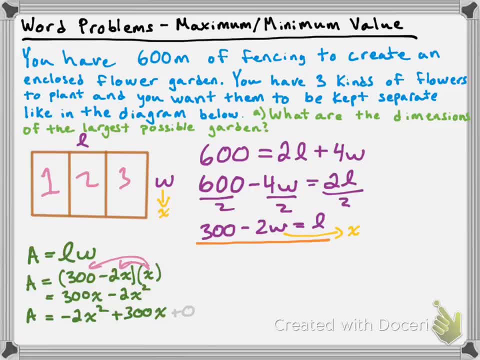 So let's do that. So there are many ways that you can find the maximum value. Remember, the goal here is to kind of find the y value of our vertex. So you could do that by completing the square and changing this into vertex form. 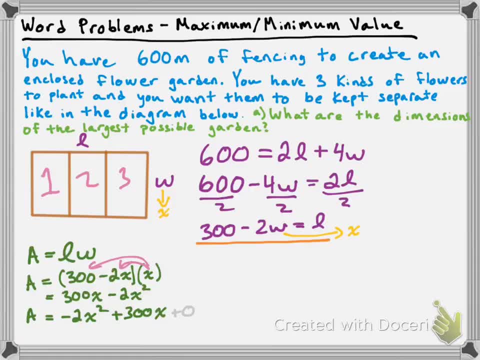 That would be an acceptable way to do this. Or you could find the two zeros, the two x-intercepts, and then average them to get your axis of symmetry and then plug your value for your axis of symmetry into the equation. Or you could do the method that I'm going to do. 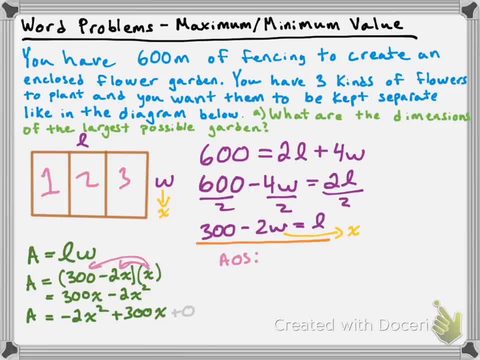 and I'm going to use the axis of symmetry formula. So the axis of symmetry formula, if you recall, is: x is equal to negative, x is equal to negative b divided by 2a. So substituting 300 for b and negative 2 in for a. 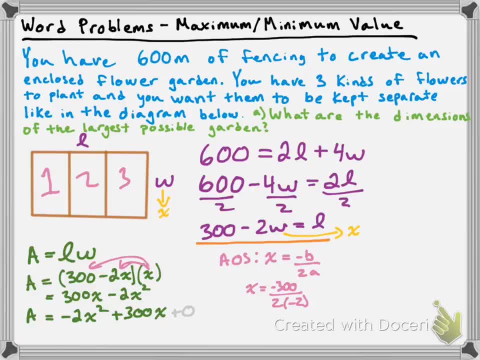 that's going to give us: x is equal to negative 300 divided by 2 times negative 2, which is negative 300, divided by negative 4, which gives me 75.. Okay, so the axis of symmetry occurs at: x equals 75. 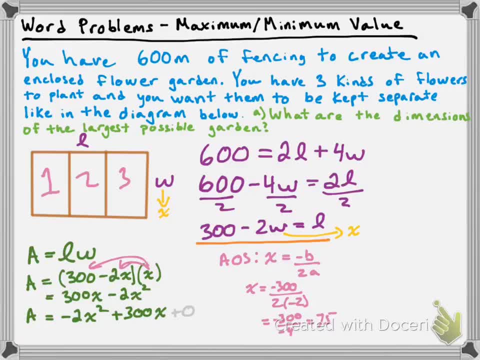 Now remember that x represents the width here. So that tells me that this x value here is the width that gives me the x value And that gives me the maximum area, because that's the x value that gives me my maximum value. Okay, so this is the width that gives me the maximum area here. 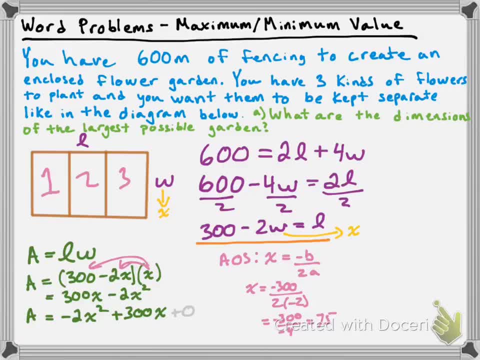 Okay, so I'm actually almost halfway done the first part of this problem: finding the dimensions, because that's the width. Now we need to find the length, But you might remember that we, conveniently, closer to the beginning of the problem, came up with a formula. 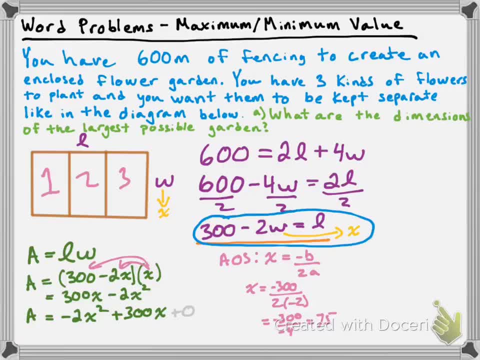 or an equation that represents the length in terms of the width. That's this guy here. So, to find out what the length is that's going to give me the maximum area, I'm going to substitute my width here. Okay, So I'm going to substitute my width here. 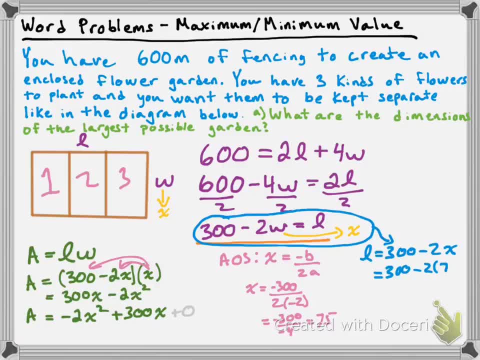 So I'm going to substitute my width in into that formula. So remember: the formula is: l is equal to 300 minus 2x. So substituting x equals 75 in for my x value, it gives me 300 minus 2 times 75, which gives me 300 minus 150,. 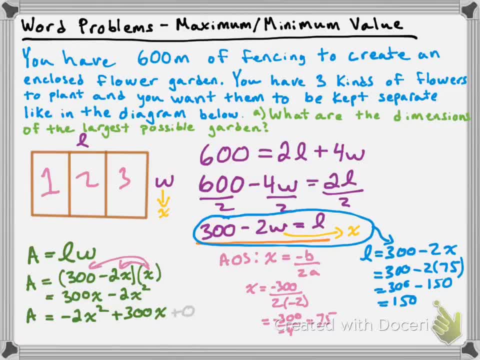 which just gives me 150.. So I know that the width for my maximum area is going to be 75 meters and the length for my maximum area is going to be 150 meters. So the answer to the first part of the question. 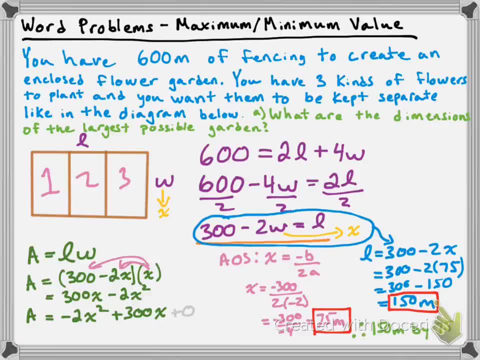 what are the dimensions for the largest possible area? Well, the dimensions are going to be 150 meters by 75 meters. Okay, so that's the kind of bulk of this question, But there is one more thing I want to discuss. Okay, so let's take a look at the next question I want to discuss. 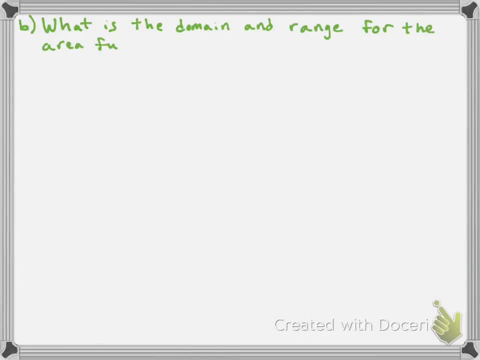 And that is what is the domain and range for the area function that we created. Okay, so what's the area function that we created? Well, remember, it's a equals negative 2x squared plus 300x. That's the one that we ended up creating in this question. 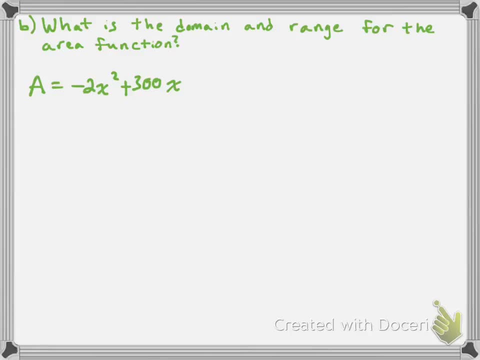 That's the equation that models the area. So what is the domain and range for the area function? Okay, in this case. Okay, so you might be tempted to say that the domain for this is going to be all real numbers, because it is. 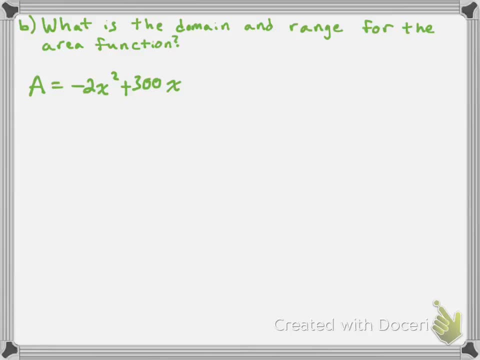 a parabola. it's a quadratic function, But you do need to remember that, since this is a real world scenario, that means that there's going to be some values for width that don't make any sense. So, for example, we know that our width could not possibly be negative 50,, for example. 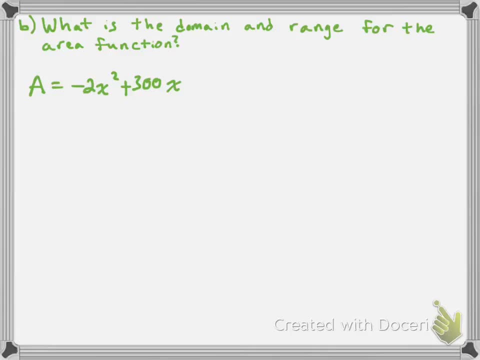 because that's just crazy, You can't have a negative width. Okay so we're going to take a look at what this looks like then. Okay so I'm going to draw out a little bit of a graph here. Okay so we have our x and y axes, which I'm going to label with: 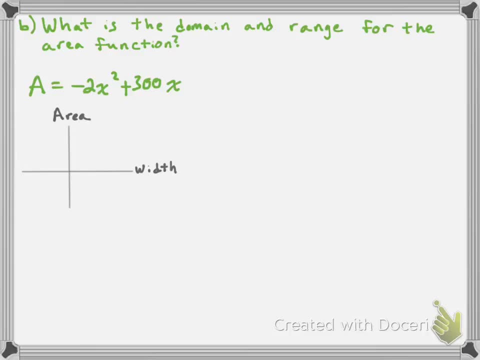 area and width. Okay, so area is our y values, essentially, and width is our x values. Okay, and we know, according to what we just did, that the maximum area is going to occur with the width of 75 meters. Okay, so I know that my vertex is: 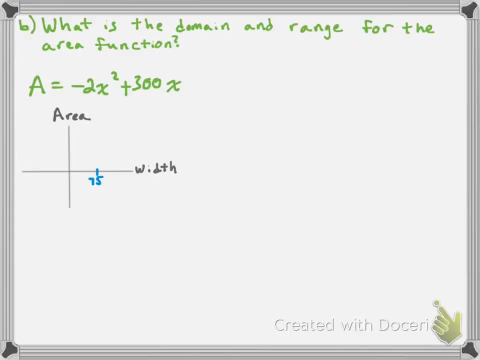 going to occur over 75, right, so it's going to be a point over a width of 75.. But we need to actually figure out what that maximum area is going to be to place my point, Because I don't know how high, to put it right now. So how are we going to find the 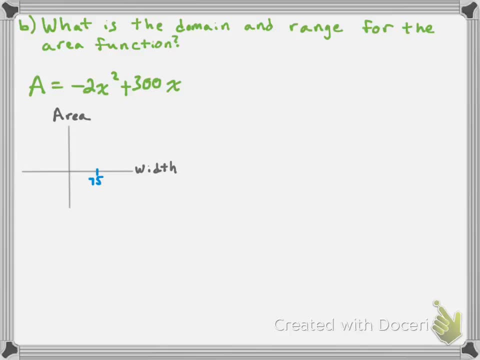 area, the maximum area. Well, we know that the width that gives our maximum area is 75.. We have an equation that represents the area given the width, so we're just going to substitute 75 into the area equation. So a is going to be. 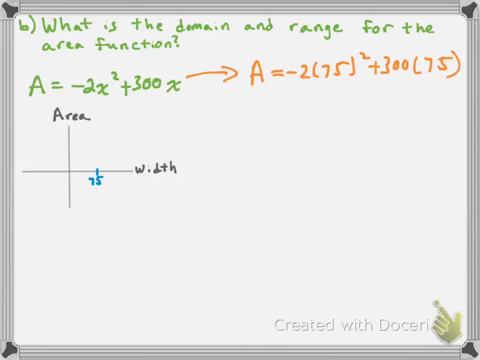 equal to negative 2 times 75 squared, plus 300 times 75.. Okay, simplifying this up, we get negative 11,250 plus 22,500, which is going to give us 11,250 meters squared. Okay, so that means that the area that's going to be the maximum area for this enclosure 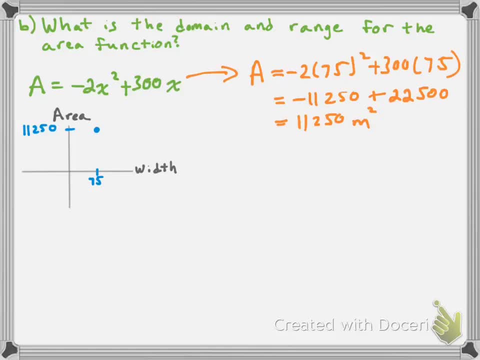 is going to occur at 11,250, so I'm going to place a point, which is going to be my vertex, over 75 and next to 11,250.. Okay, so that's pretty good. so far We got our vertex, but 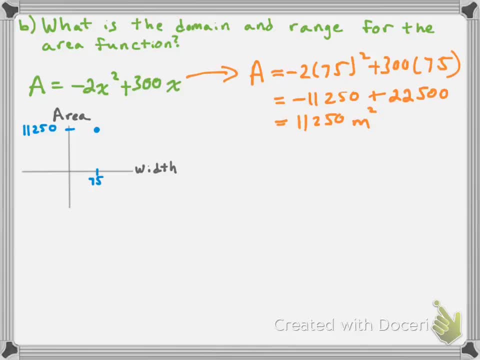 that's not really going to be enough to state the domain and range, is it So what we're going to need now is at least a couple other points. So what I'm going to do is I'm going to find the two x-intercepts or, I guess, the width intercepts. 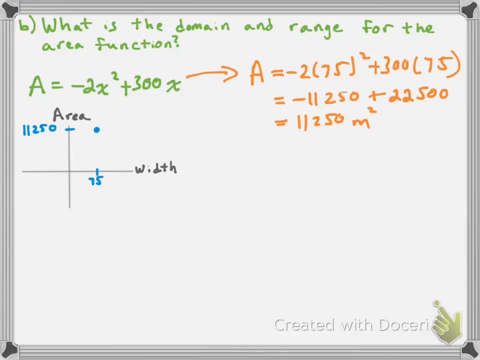 so to speak, of our function. and I'll plot those. And the easiest way to do that would probably be to factor in this case. So let's factor the equation. So if I factor it, let's see I can pull out. 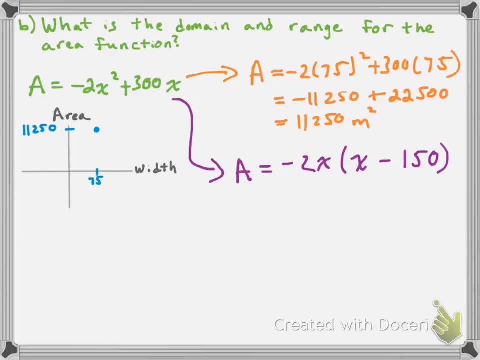 a common factor of negative 2x. so that gives me a equals negative 2x times x minus 150.. Okay, that's fully factored. So that tells me that something times something is going to be equal to area. and if my area is going to be 0, because I am looking for- 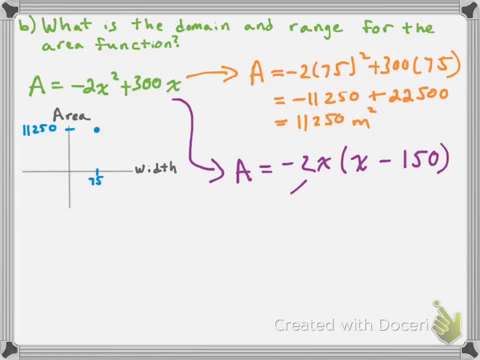 the x-intercepts, and that's where my area is 0,. that tells me that I'm going to have a solution when negative 2x is equal to 0, which tells me that x will be 0 there And I'm also going to have a solution. 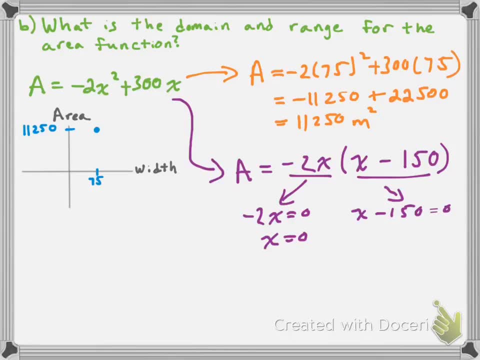 when 150 is equal to 0, and so that means my second solution is x equals 150.. So that means I can actually plot my x-intercepts or my width intercepts now, So I'm going to have one at 0. 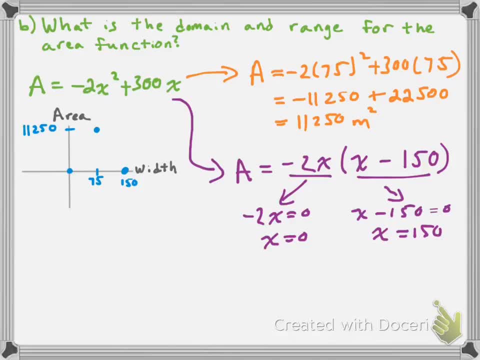 on the origin and I'm going to have one at 150.. I have three points. I'm going to just kind of sketch in a little parabola there. Okay, so there's my parabola And I want you to notice a couple things. So first of all, 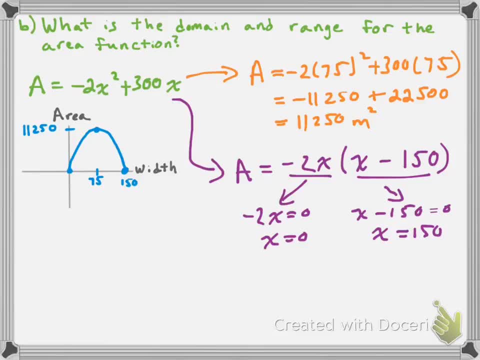 I want you to notice that I have not drawn my parabola down below the width axis. Now let's think about why that would be the case If I did draw parts of my parabola down below the width axis. that would tell. 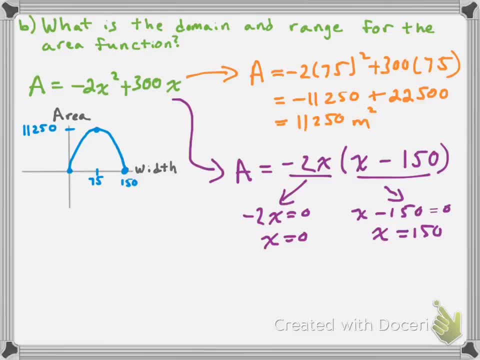 me that I would have negative area there, And we know that doesn't make any sense, so I didn't even bother drawing it. Okay, Also, notice that I do not have any points to the left. I do not have any points to the left of my area axis. 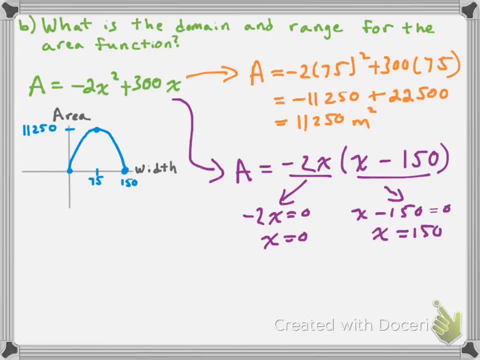 because that would imply we would have a negative width, So we leave that out as well. So this is all I'm going to draw Now. this is going to help us with the domain and range, because the domain and range are going to be slightly different, given that this is a real world scenario. 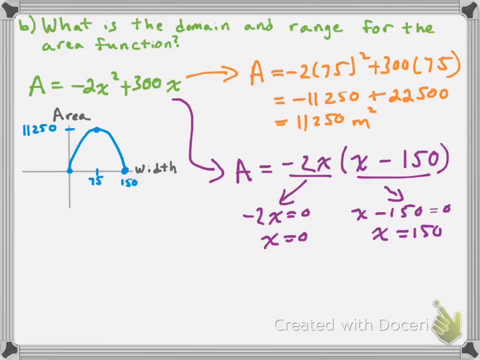 We need to have positive widths and we need to have positive areas. So, according to the sketch I made here, the domain is going to be the set of x values, which are elements of the real number system. okay, So for domain, we're talking the x values. It looks like my smallest x. 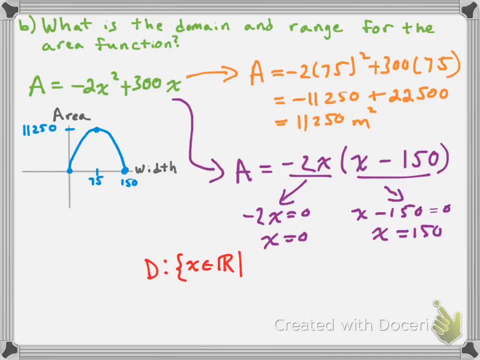 value would be at 0, and my biggest x value is going to be at 150,. okay, So I know I'm going to have values between 0 and 150.. So let's see, 0 is going to be less than x, which is going to be less than. 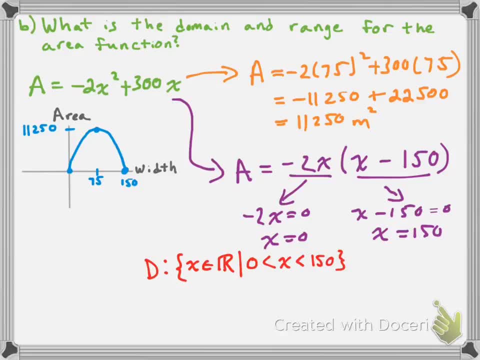 150.. Now I want you to notice that I did not actually put less than or equal to for either of these signs, And the reason why is that I'm actually preventing my closure from having 0 area, So I'm saying it could be bigger than 0,. 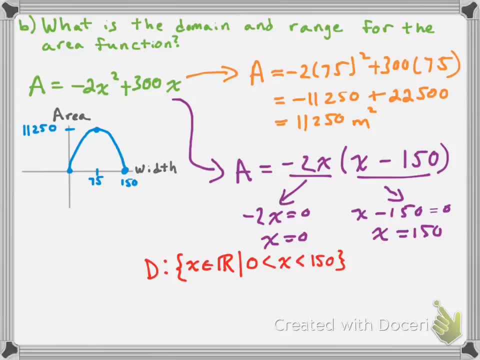 but it's not going to be equal to 0, right, I'm going to have some sort of width at all times, And I'm basically doing the same thing for the less than 150 part, because if the width was equal to 150, that would mean my length would be 0.. And again,